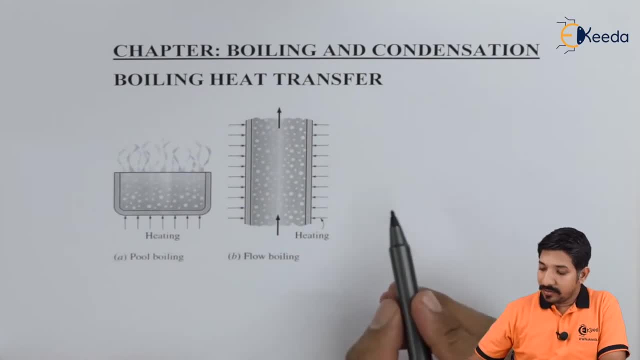 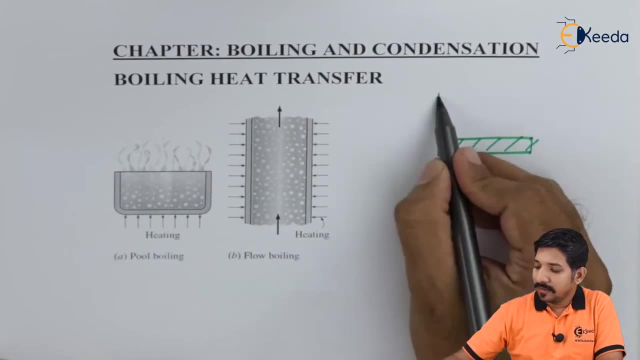 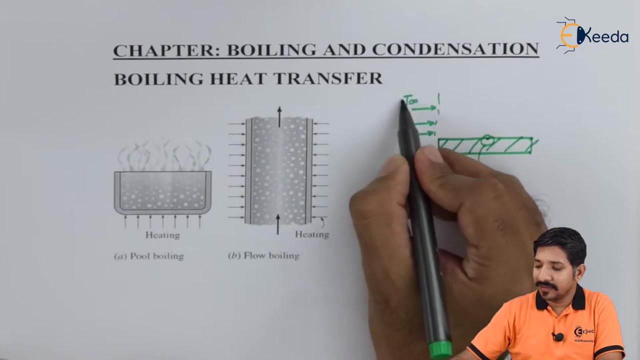 The boiling heat transfer. To describe the boiling heat transfer, let us consider a case. Let us consider a plate whose temperature is, let us say T- s, and then a fluid is flowing over a plate whose temperature is, let us say T, infinity. Now, in this case, what will happen? Obviously, 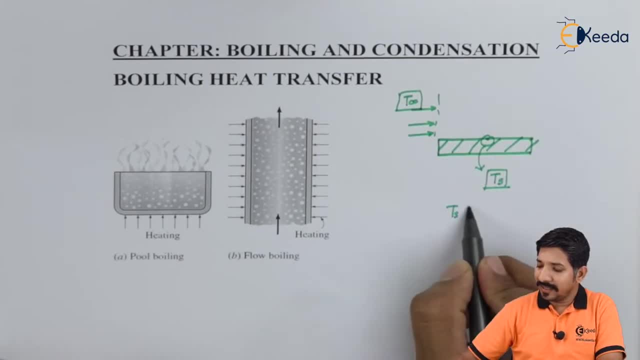 if I assume that the temperature of the plate is T s, then the temperature of the plate will be T infinity. If I assume that T s is greater than T infinity, then the heat will flow towards the fluid. So then, what kind of heat transfer will be there? Obviously, for the first. 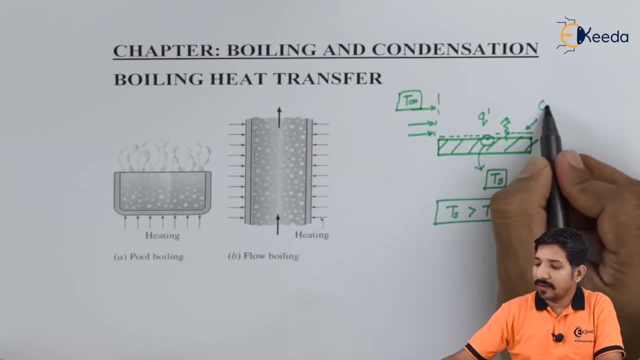 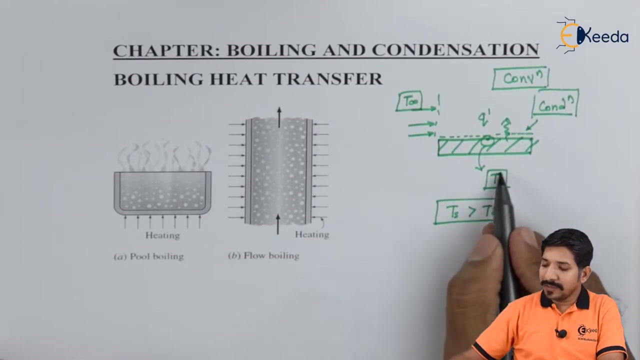 layer, we will have conduction and then after that we will have a convection. Now question need to be asked that what should be the temperature till which the conduction and convection will take place? Now, to answer this, we need to understand the T s diagram. 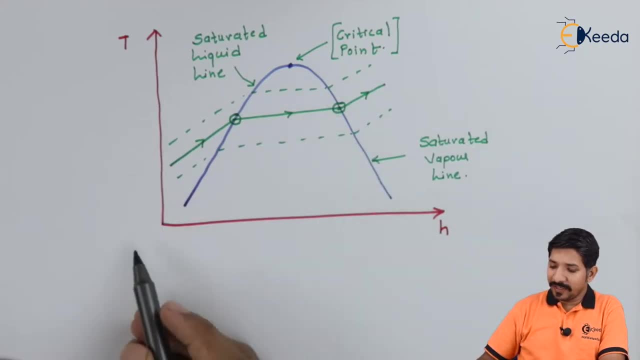 Let us understand this T s diagram. Now, in this T s diagram, what we have done? we have simply kept a water whose temperature is, let us say, 30 degree Celsius. And if I keep on heating this water, what will happen? Obviously, let us say, if I assume that 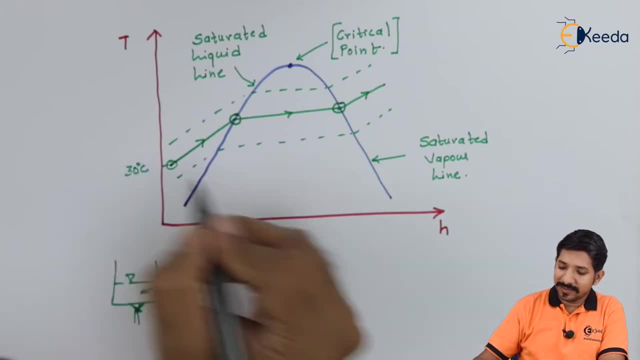 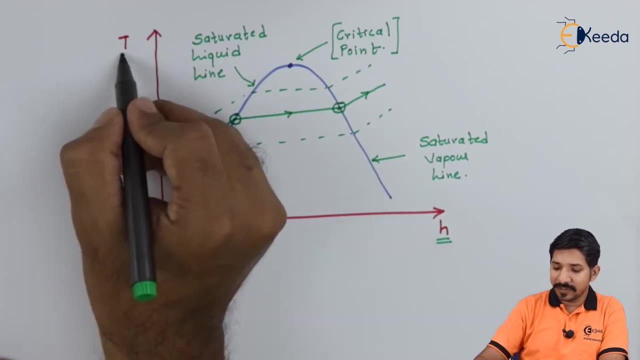 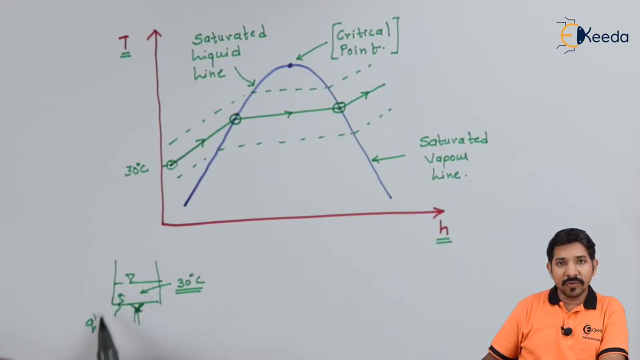 this temperature corresponds to 30 degree Celsius. then if I keep on heating, it means my enthalpy. So basically, this diagram indicates temperature versus enthalpy. If I keep on giving heat to the system, what do? what is going to happen? The enthalpy is going to change. 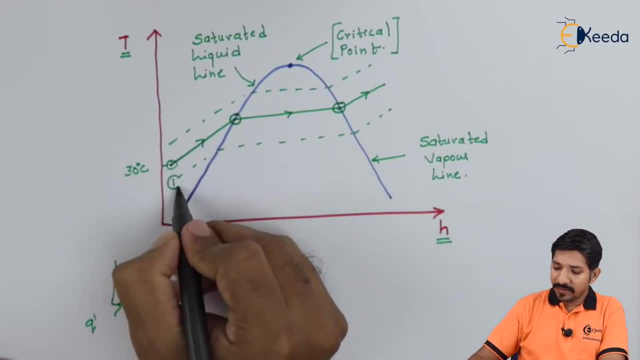 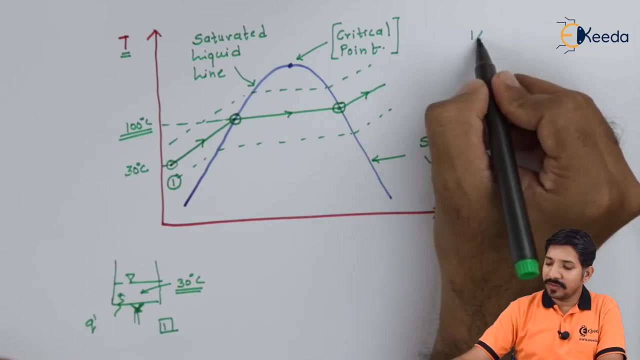 So let's say, from point 1, where this indicates point 1, the heat is given to the fluid and fluid is reached to a state that is 100 degree Celsius and we all know that for one atmosphere, 1 atm, that is one atmospheric pressure which we know is one bar, approximately one bar at 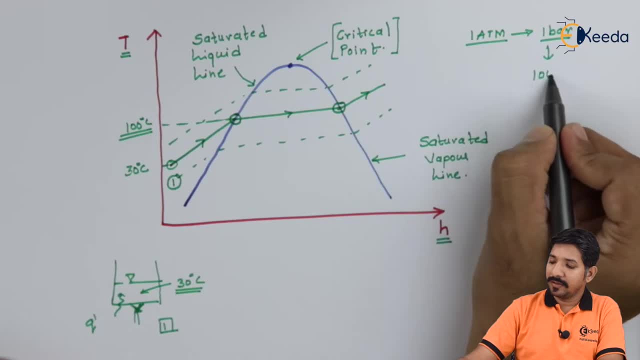 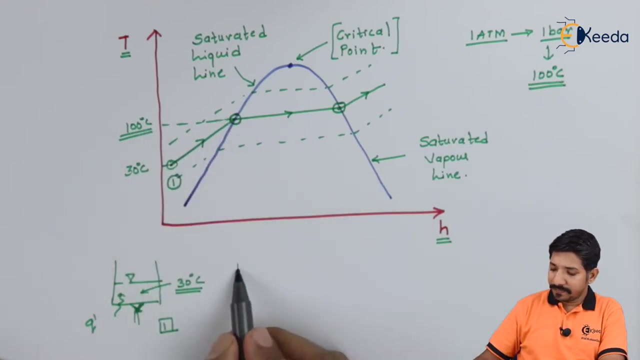 one bar. my saturation temperature is 100 degree Celsius. although it is not 100, it is approximately 99.97, but for sake of simplicity, let us consider this as 100 degree Celsius. now, as soon as I reach the 100 degree Celsius, what is going to happen? so again, if I assume that this is, 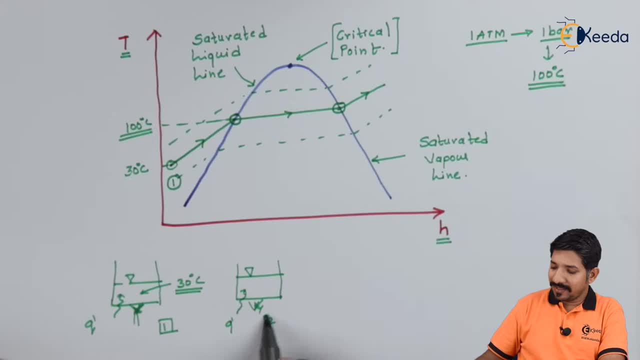 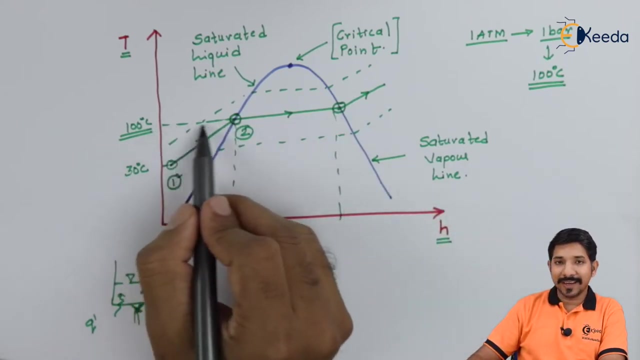 a fluid. So let us say that This has state number 3 and this is kept at 100 degree Celsius. so what will happen after that? now, even after point 2, if I keep on giving heat, the temperature will not change till certain point. okay, now, in this case, my temperature remains at 100 degree Celsius till entire. 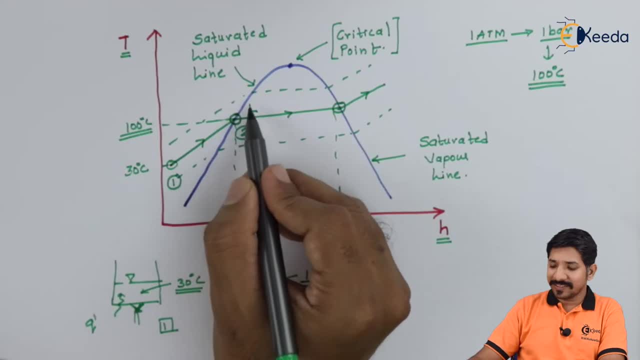 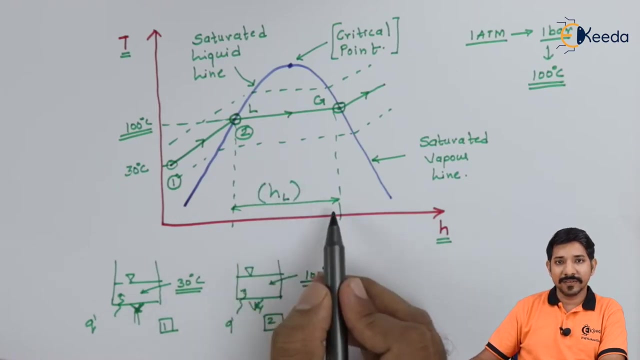 liquid or entire water. in the liquid state it is getting converted into a vapor, Vapor state or a gaseous state. so this enthalpy is what they call as enthalpy of, or latent heat of enthalpy LH. then, once it reached to a 100 degree Celsius gas, and even if I keep on increasing 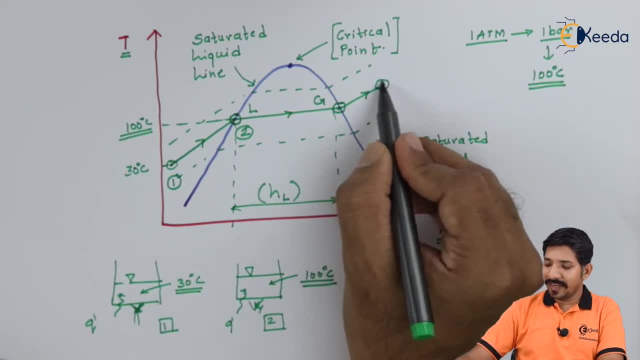 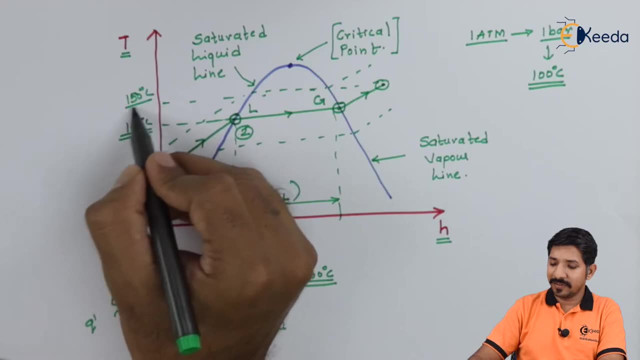 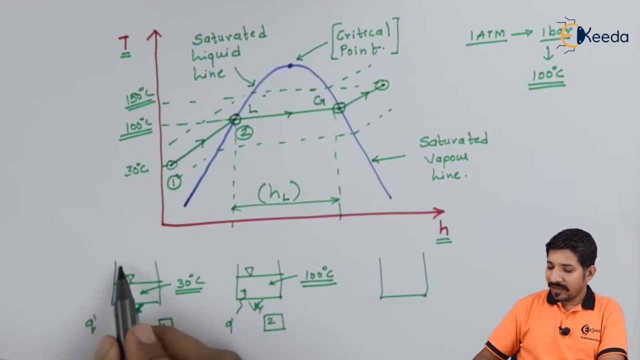 then what will happen? then the temperature will increase. so let's say, if I reach to a point Where the temperature is 150 degree Celsius, Okay, Okay, Okay, Okay, Okay. So at 1 bar 150 degree Celsius, we will have a vapor. so in this case, if I consider this, 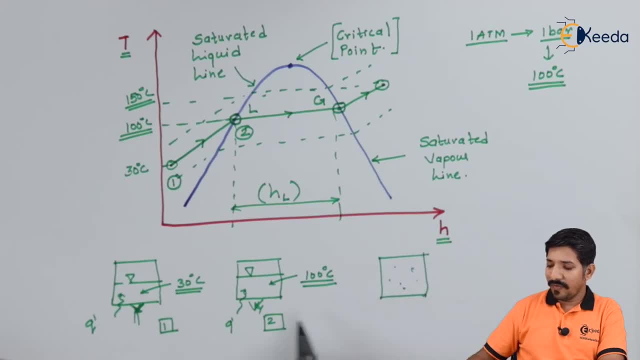 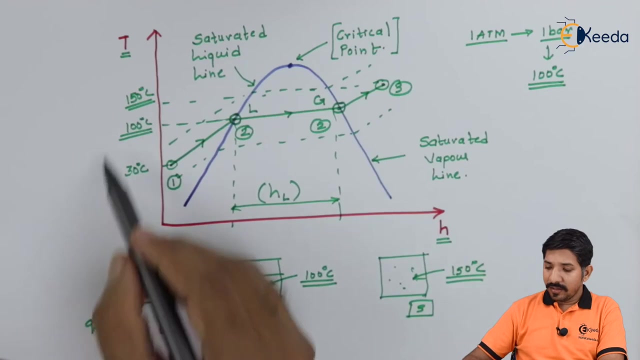 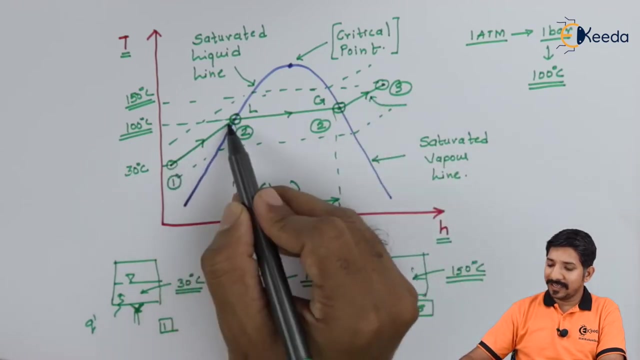 as a closed container, then we will only have a vapor over here. So why am I explaining this thing? this thing we have done previously, but the purpose of explaining this thing was to make you understand that this way the curve will be formed. now this is done for a one ATM, so this entire curve is plotted for one ATM or one bar. now. 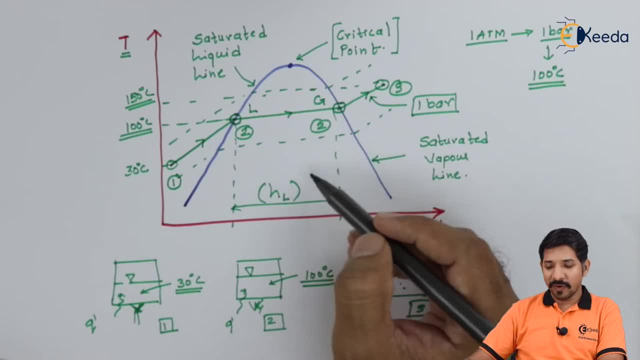 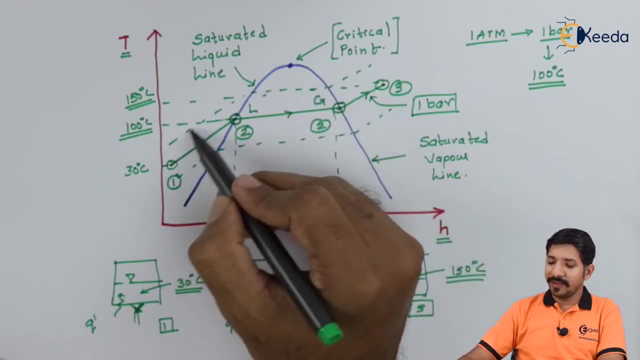 similarly, if I keep on reducing the pressure, what will happen? the line will come something like this: this ordered line. or if I keep on increasing the pressure, the line will come something like this: now, if I try to plot this kind of curve for all the ranges of pressure, 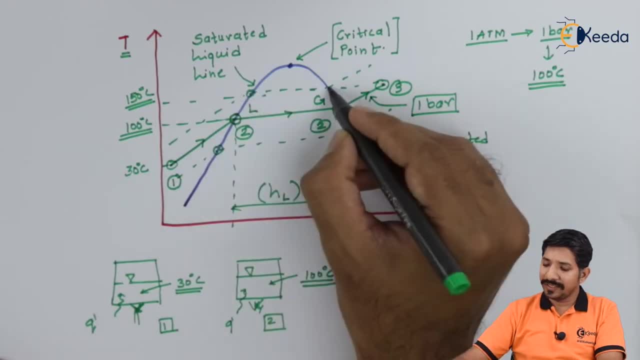 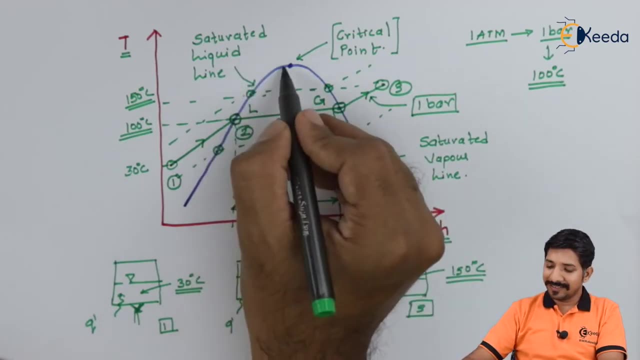 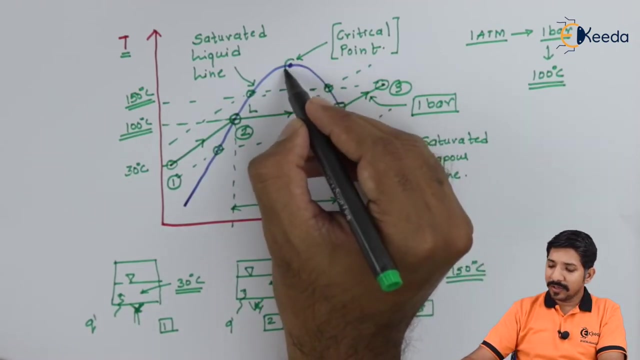 and If I start joining these points, we are going to end up getting this kind of curve. now this kind of curve is what they call as a saturation curve. now, this line is a saturation liquid line and this line indicate the saturation vapor line and this point is what they call. 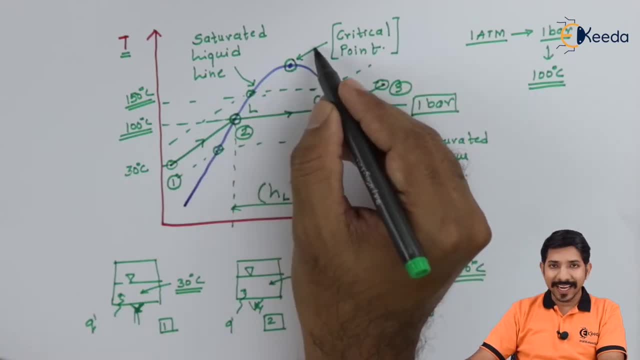 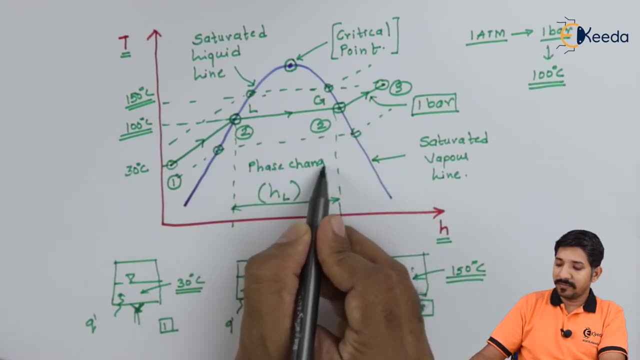 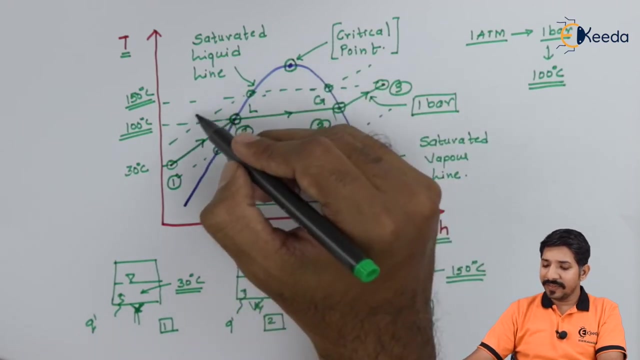 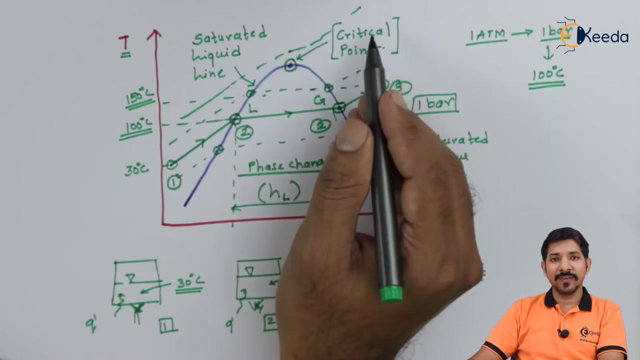 as a critical point. why is it so? because after that there is no phase change, so this part they call as a phase change. Okay, After this point, if I keep on increasing the pressure and temperature, there won't be any phase change. the The liquid to gas vapor transition will occur suddenly. 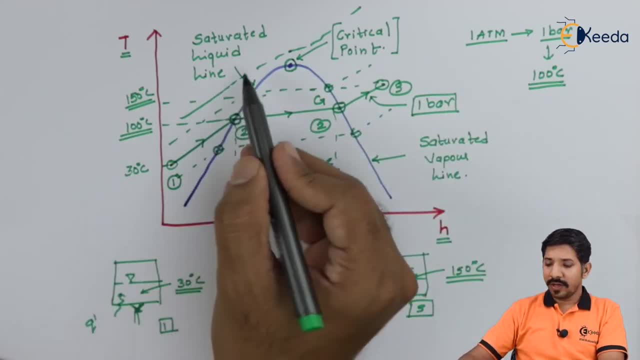 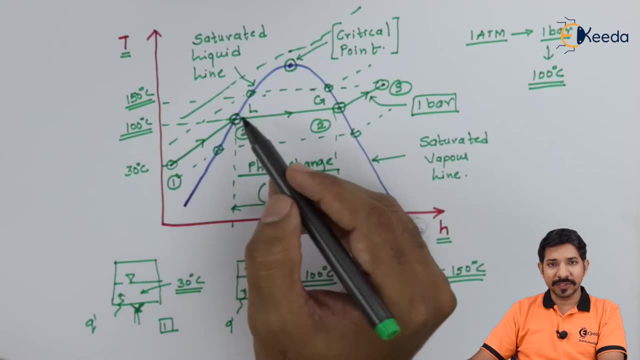 So the purpose of explaining this thing is to make you understand what do you mean by the saturation liquid line and what do you mean by the saturation vapor line and basically what is the saturation temperature. So for one bar, my saturation temperature was 100 degrees Celsius. 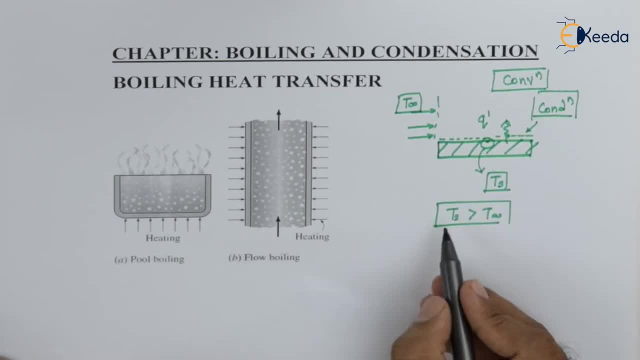 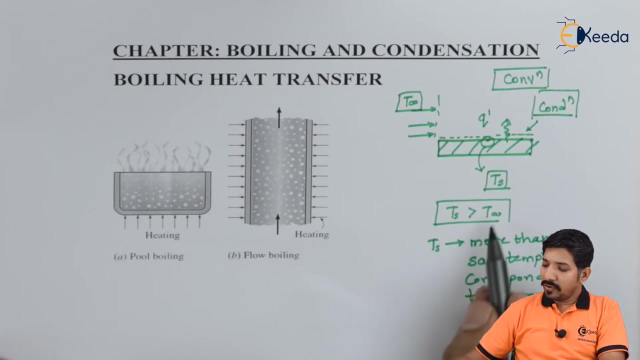 Okay, Now, with that you can understand if my TS becomes more than saturation temperature corresponding to its pressure. If this is the scenario, then the boiling will surely take place. So in this case, as the temperature or as the TS started increasing, initially the conduction 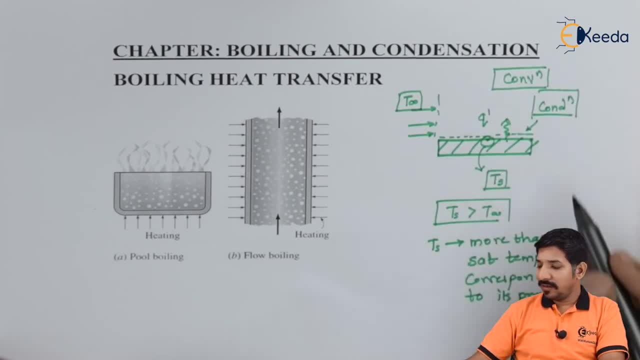 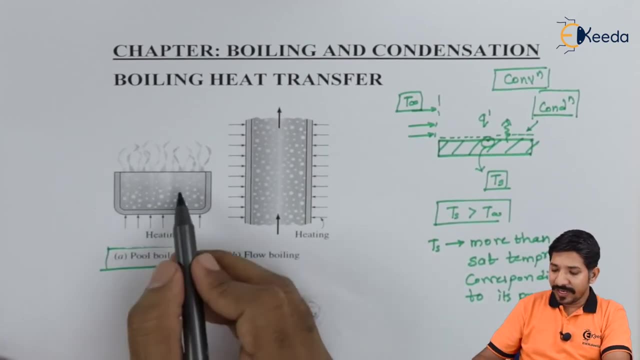 will take place, then the convection and then, obviously, the boiling will take place. There are three types of boiling. one is a pool boiling, where a fluid is kept inside a vessel and there is no movement. there is no external movement of the fluid. so, whatever the movement of the fluid, 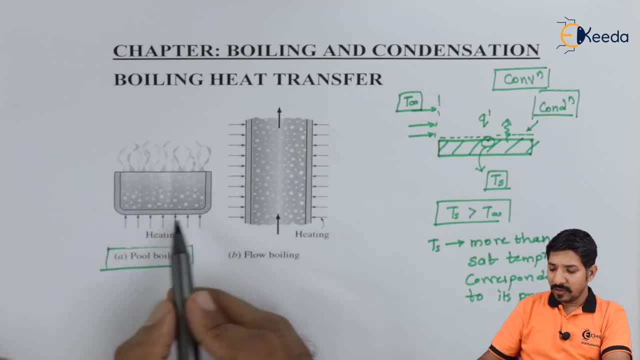 That takes place is by the buoyant force. it is So all the bubbles that are formed. they will carry themselves upward and then the space will be filled by the colder fluid. So this kind of boiling is nothing but the pool boiling. The best example is FBTR. 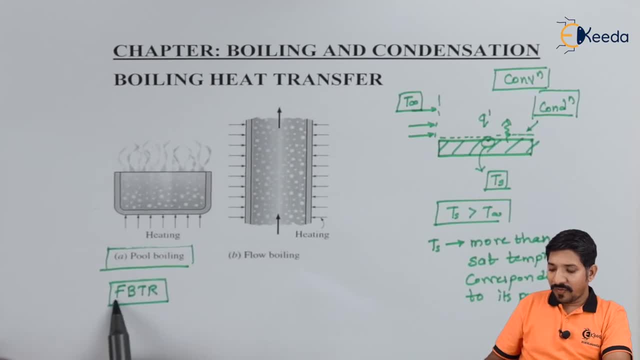 So that is fast breeder test reactor. Now this is a nuclear power plant. In this nuclear power plant The core is kept inside the molten metal fluid and the cooling will be taken place by the liquid molten metal fluid. to understand the heat transfer rate in case of a FBTR, we must 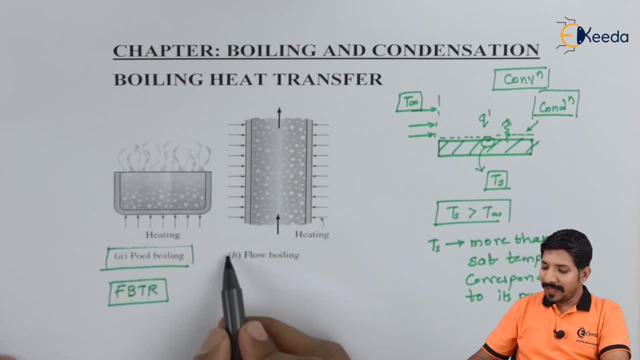 understand the pool boiling Similarly. the second is flow boiling. Now flow boiling, again instrument can be kept vertical or horizontal. Now in this, obviously, there is some external agent is used, such as pump or blower, to flow the, to make the flow of the fluid. 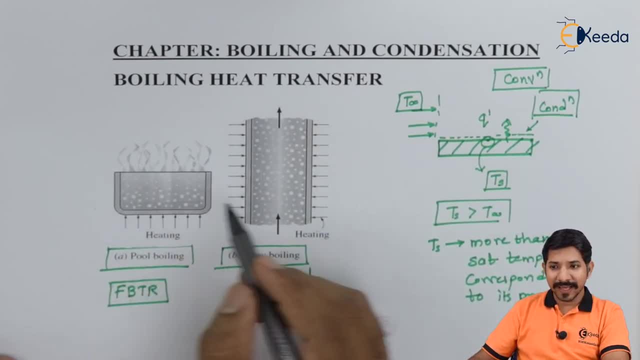 So basically the fluid motion will be driven by the buoyant force and some external agent. Now in this case the size of the bubble formation will depend on the velocity factor. also, there is no velocity factor in case of a pool boiling, So obviously one can surely make it out. 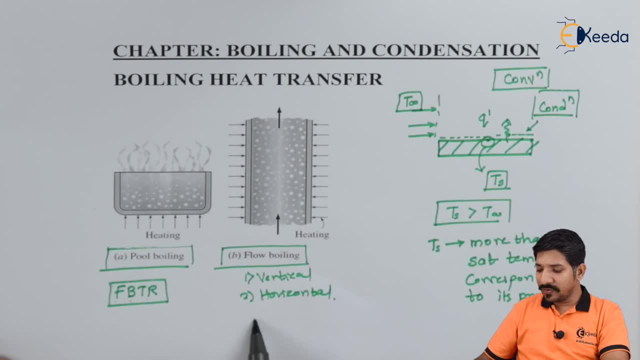 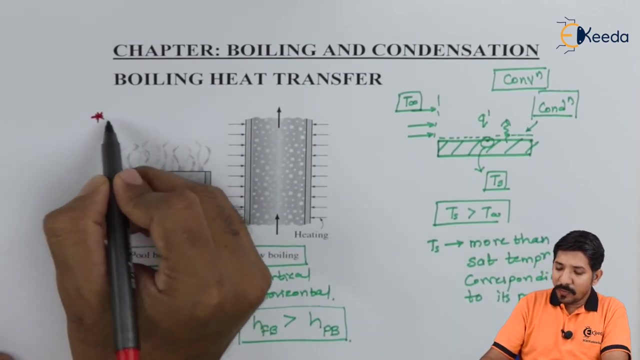 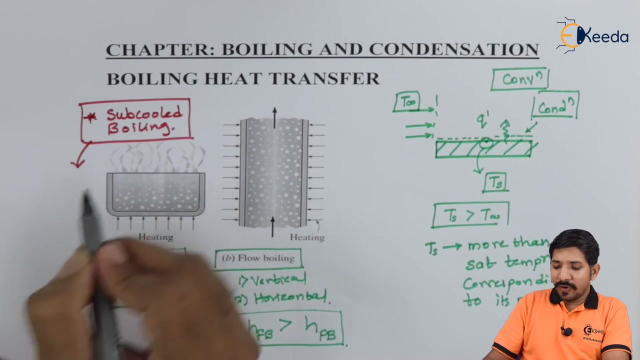 That The heat transfer rate or the heat transfer coefficient in case of a flow boiling is quite higher as compared to the heat transfer coefficient in case of a pool boiling. Apart from these two, there is something called a subcooled boiling. See, in case of subcooled boiling, the surface temperature may not be equal to or may not. 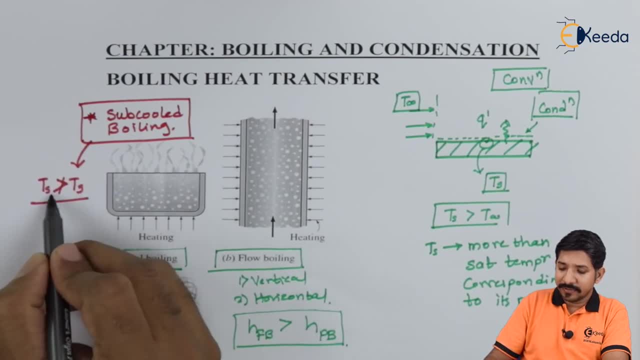 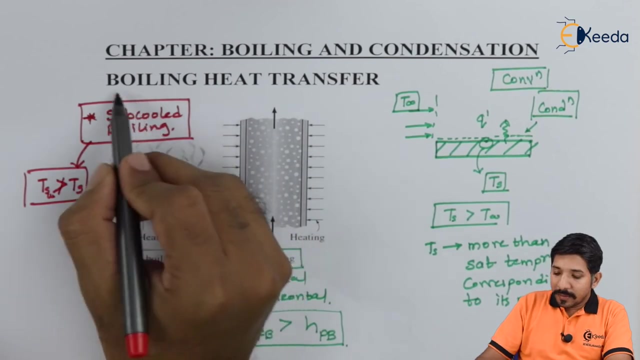 be more than The Saturation temperature. So the surface temperature is less than the saturation temperature. So the bubbles will be formed very near to the surface. but those bubbles will never be carried out. Those bubbles will die on the surface itself. The boiling. 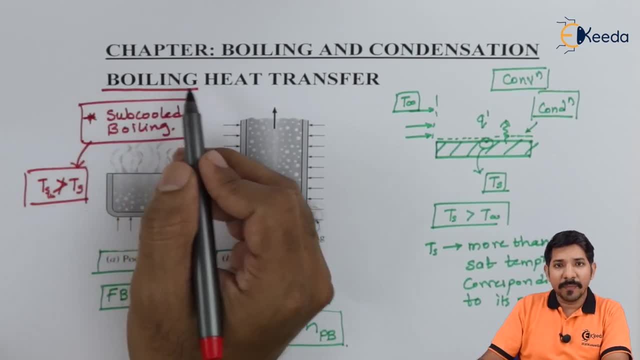 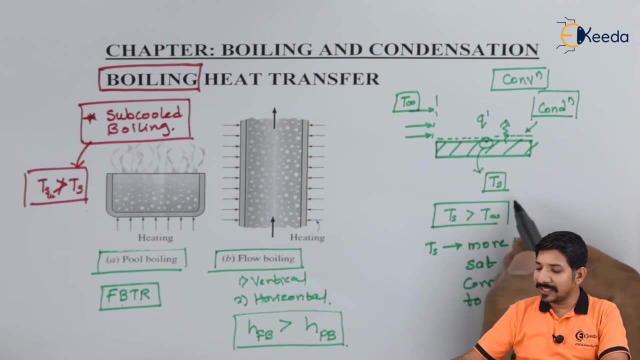 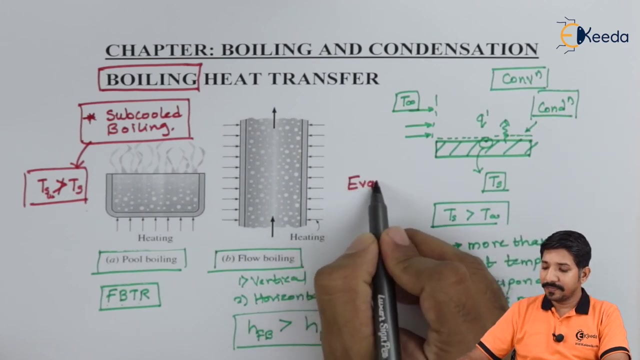 There is a difference between the boiling and evaporation. What do you mean by boiling? In case of a boiling, my temperature reaches to a saturation temperature and then the boiling takes place. So the question is ask: what do you mean by the evaporation? 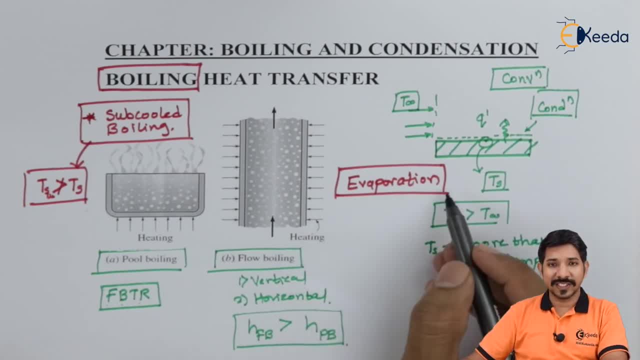 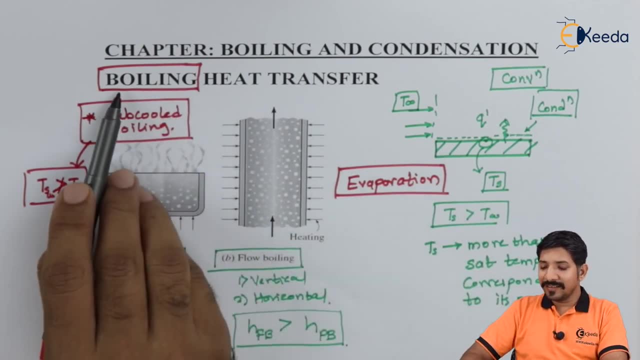 Because in both the cases the heat will be transferred because of the phase change. In boiling there is a phase change, so is there is a phase change in the evaporation. But what is the difference? The difference is: in boiling the temperature reaches to saturation temperature. in evaporation,